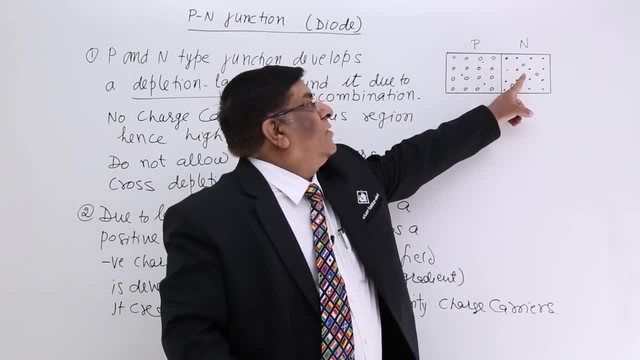 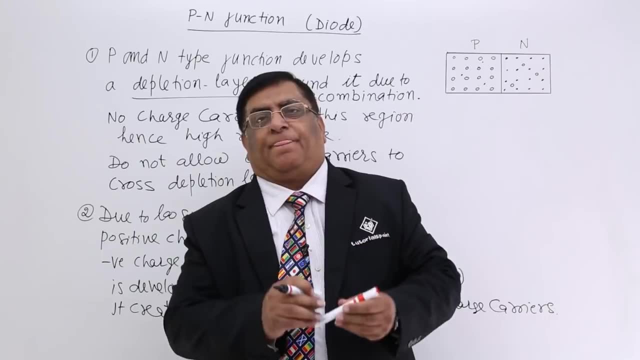 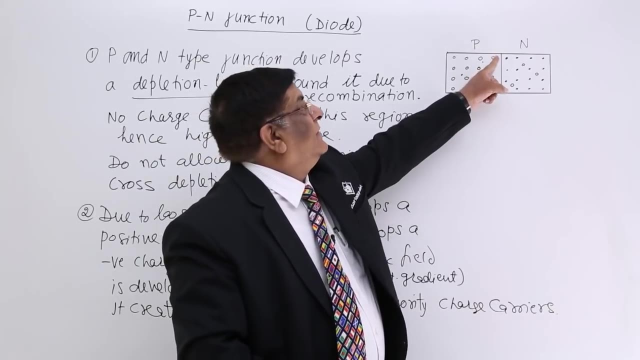 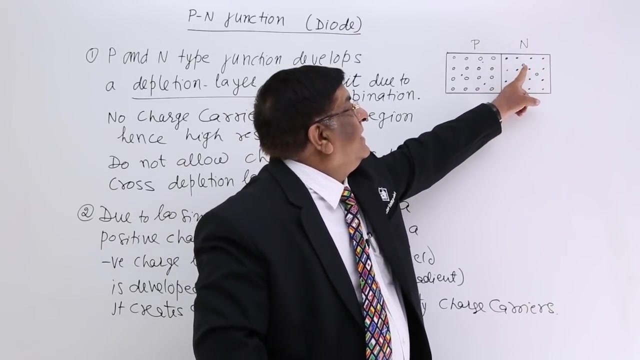 Here is a block of p-type semiconductor and a block of n-type semiconductor and we are joining the two blocks this way. When we join the two blocks, what are in majority? in p-type, The holes are majority charge carriers and in n-type, electrons are majority charge carriers. 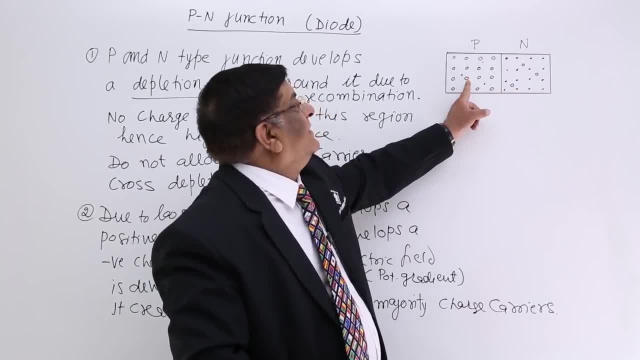 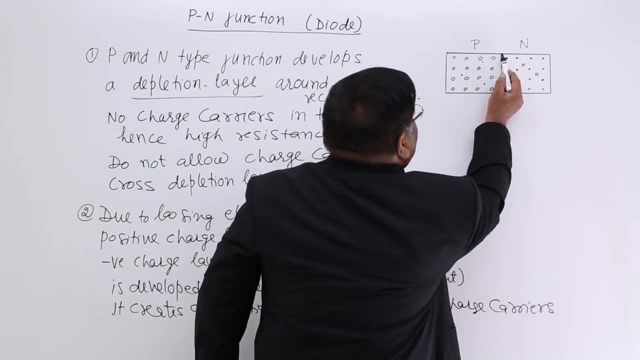 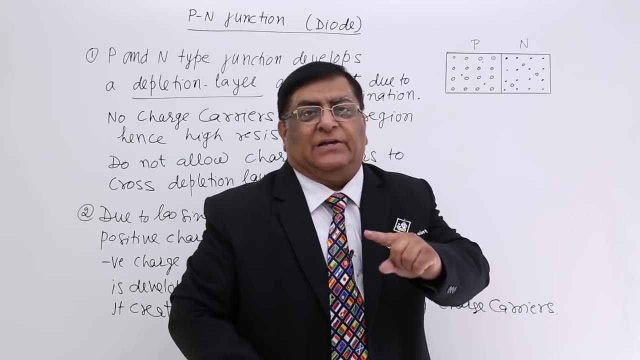 There are certain holes as minority charge carriers Here in p-type these are electrons which are minority charge carriers. Now, when we join the two, this is the junction and what happens across the junction The moment we join immediately. one current start: What? 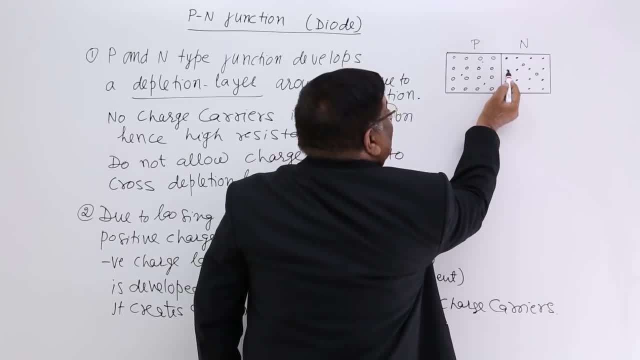 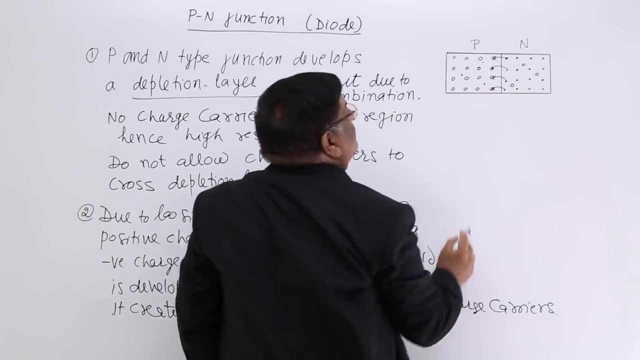 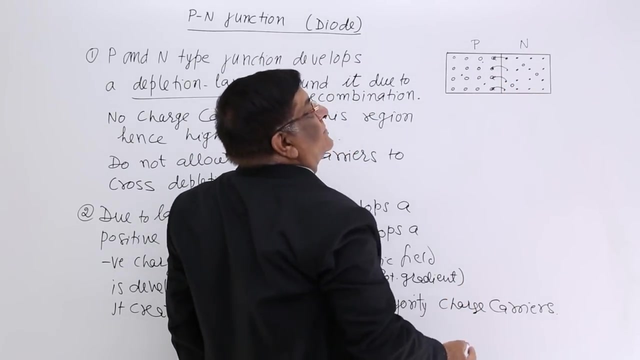 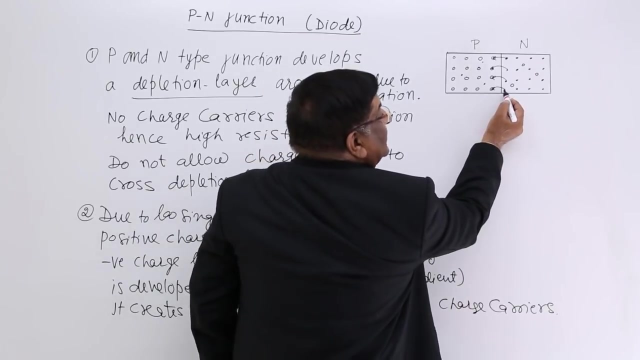 is that current, This electron, attracted by this positive charge, jump here, Okay, And because of this current, there is neutralization of this hole. Due to this neutralization, this electron is consumed. so there is no charge at this location There. 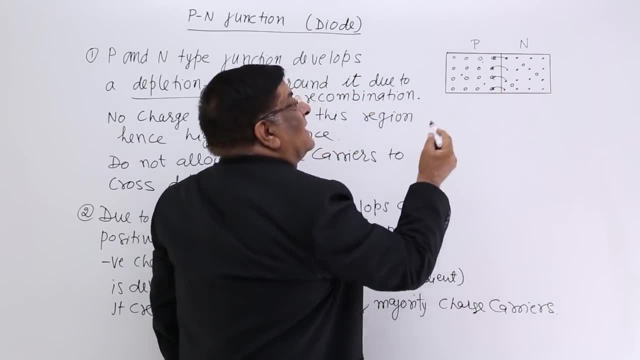 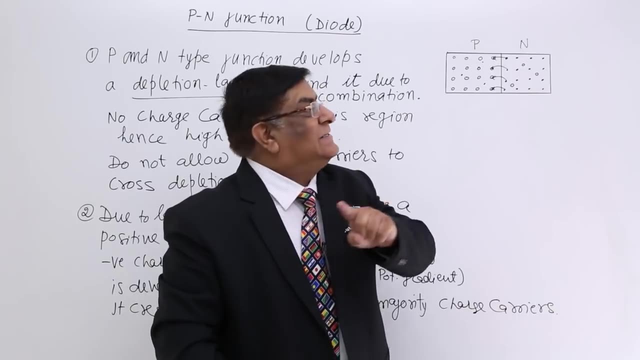 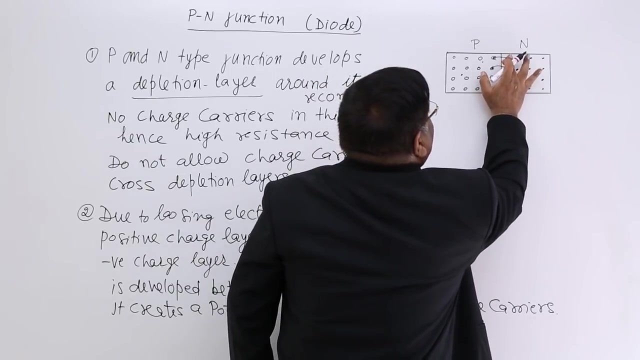 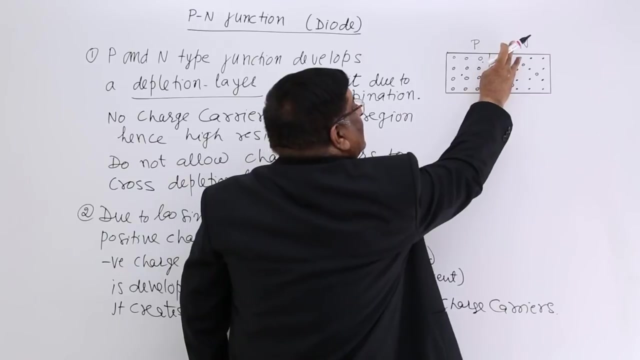 is no charge at this location, because this plus has become zero, this minus has become zero. So, after this current, what is the final situation? Answer: final situation is that here we have a layer and that layer has 2 borders: One border here and one border here. What has happened here? All the electrons have mixed. 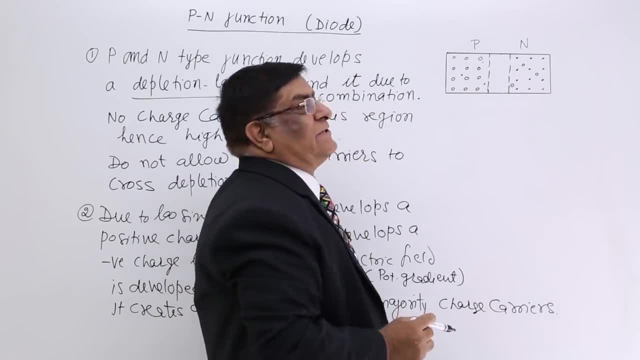 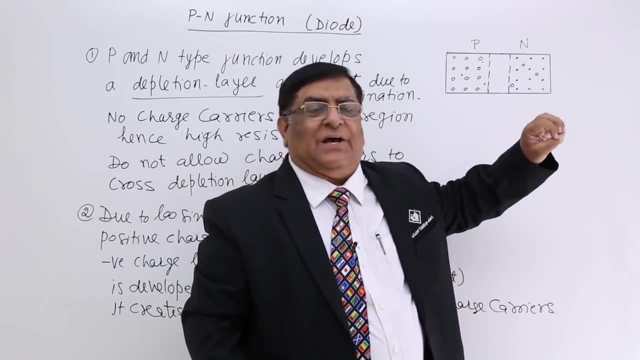 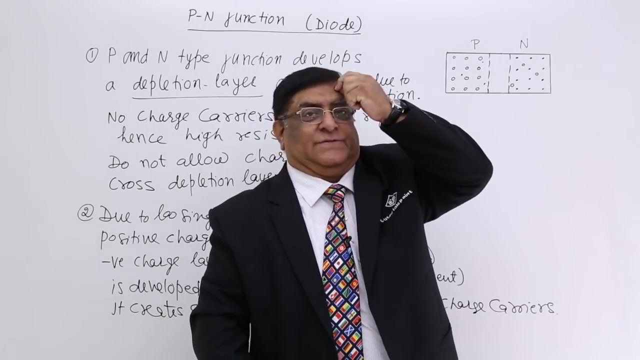 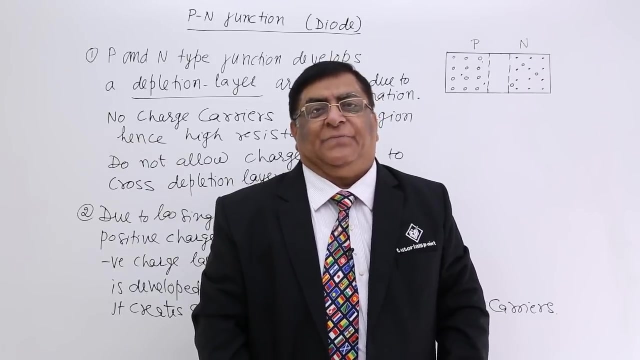 with the holes, Okay, OK, have become complete atoms and those electrons are gone. so there, only atoms are remaining, whatever are there in this semiconductor, but there are no free electrons. so there is this layer which is not having any charge carrier. now, if this layer is not having any charge, 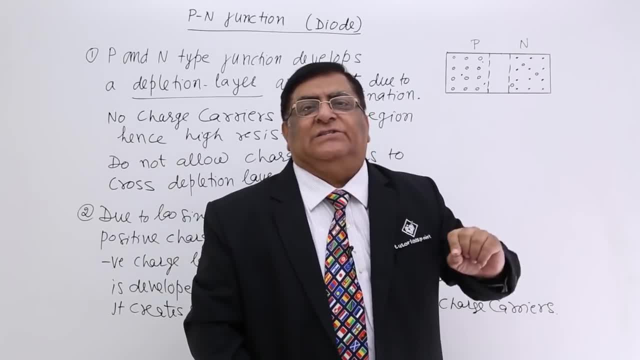 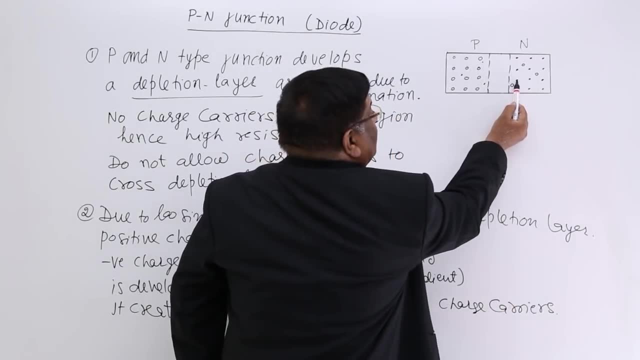 carrier. we give it a name because the charge carriers have depleted. we call it depletion layer. now this electron wish to go and utilize this hole. but this is a large resistance and you know how electron moves: it goes to one positive charge, then it jumps to other, then 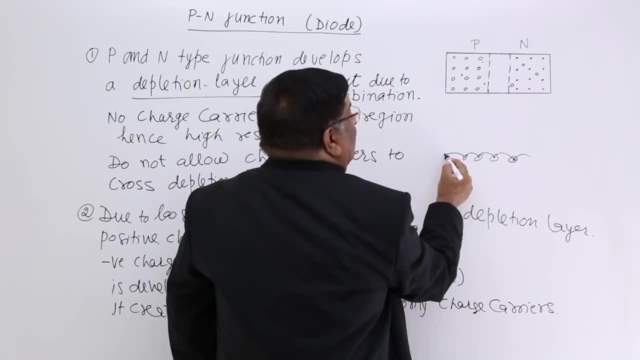 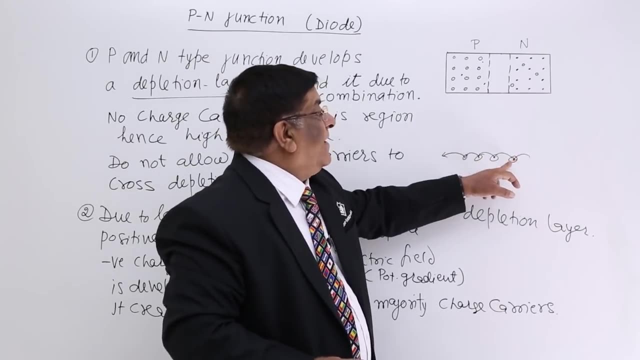 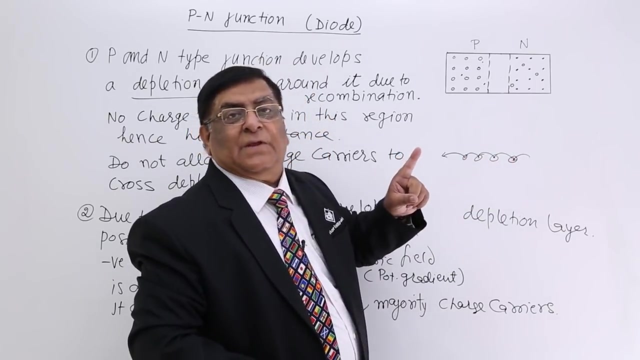 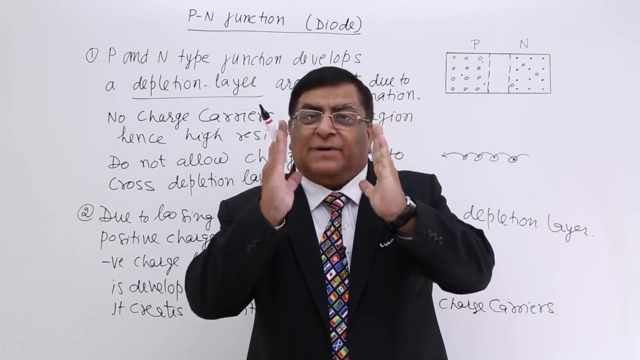 it jumps to third, then it jumps to fourth and it come here. this is the way how it moves. an electron would like to move. for him, the hopping is a easy manner. so what he needs, he needs this charge particles. so for any place, if charges has to move, then this place. 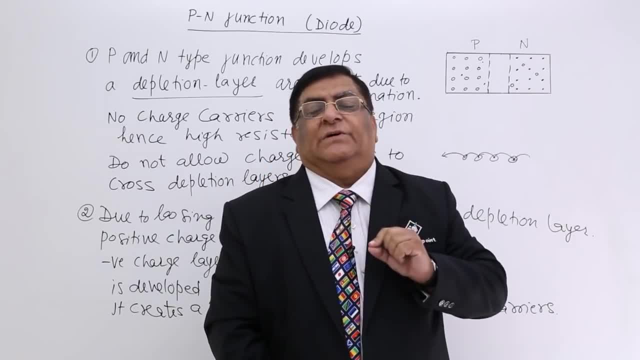 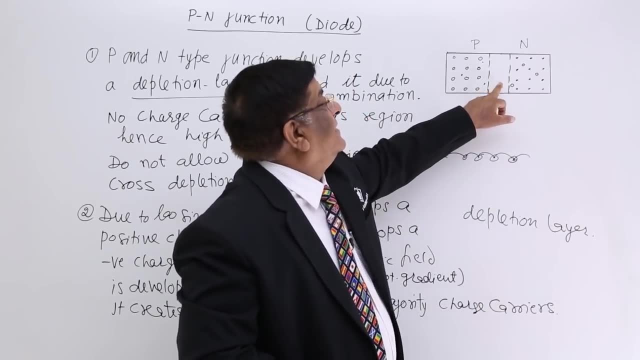 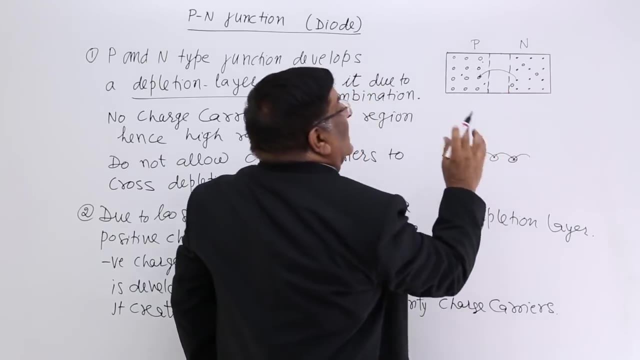 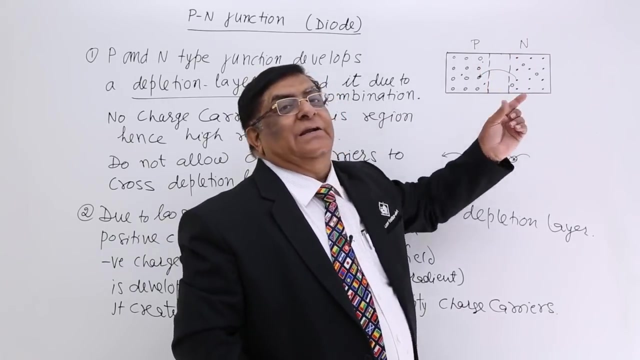 must be having charge carriers which will move. that is how the charge carrier will keep moving. if there is no charge carrier here, then this electron should have a very large energy to make such a large jump. and it is not having that. if it is having that, it will make it, it will make it, it will make it, and then we. 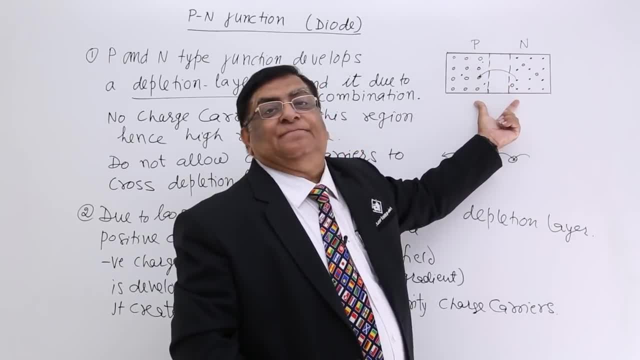 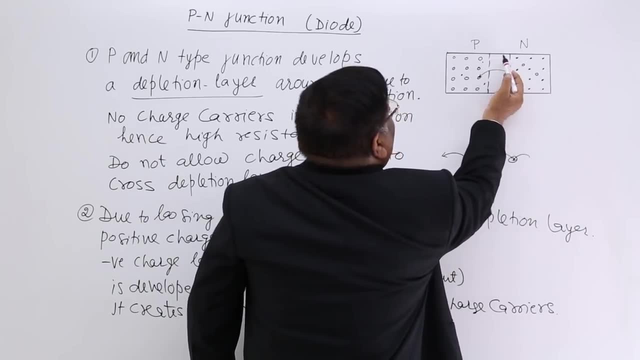 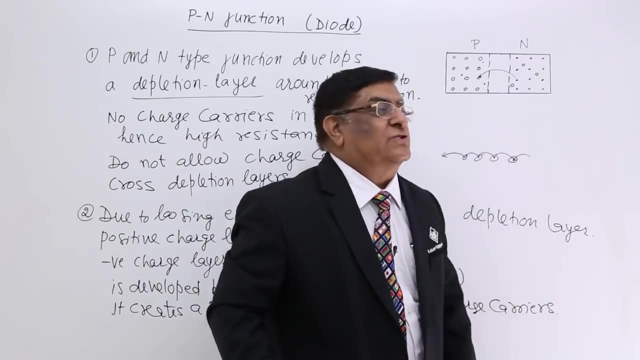 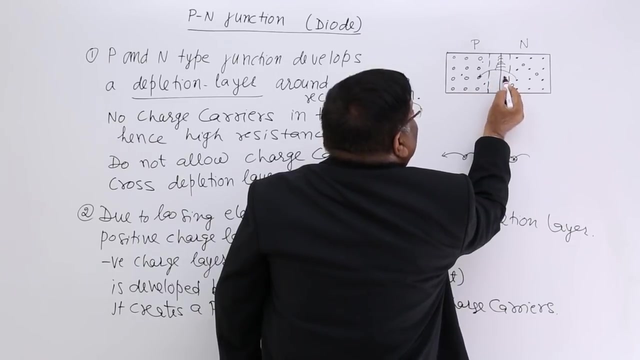 have a depletion layer this large, after that, ok, the depletion layer will be here, and after that this electron cannot jump this, so that will become the depletion layer. the charge carrier, the current in any case, will stop. initially here, this jump here, then this jump here, then this jump here and now this cannot jump here, so it stopped here and this is the. 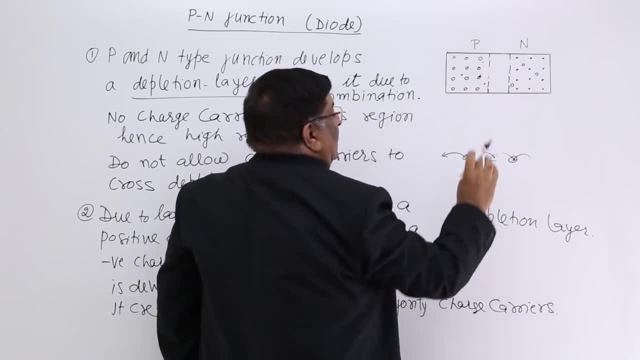 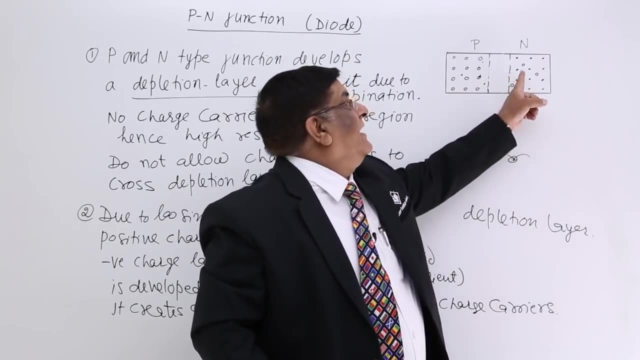 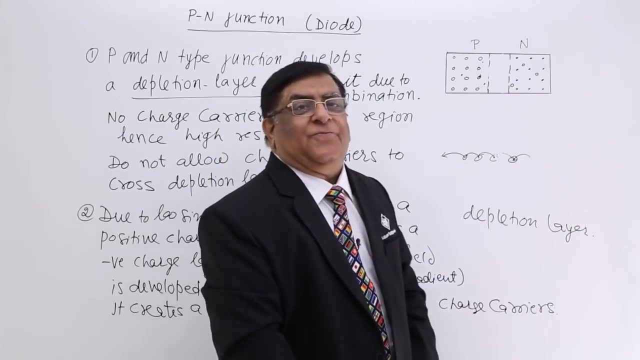 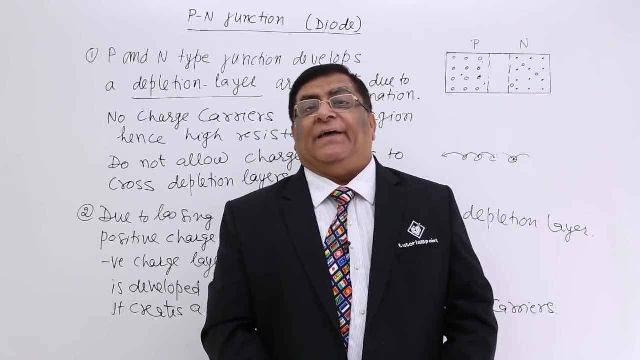 depletion layer. now these electrons cannot jump here. so what happens? a depletion layer develops in this. there are no charge carrier, no further current can flow in this layer. ok, that is one thing happens. and if current cannot flow through a reason, what we call, we say, it has got a resistance, a very high resistance, so we can say a resistance. 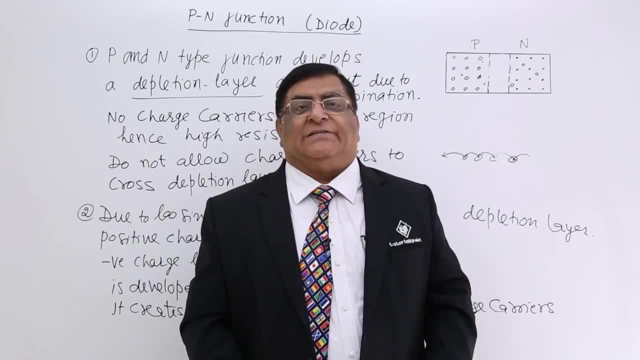 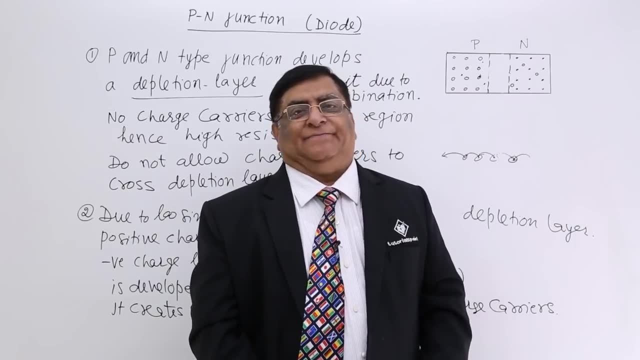 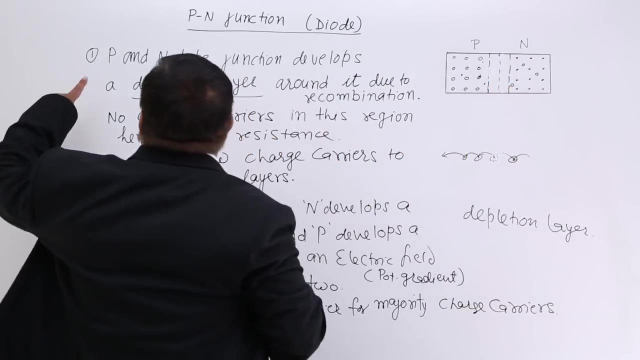 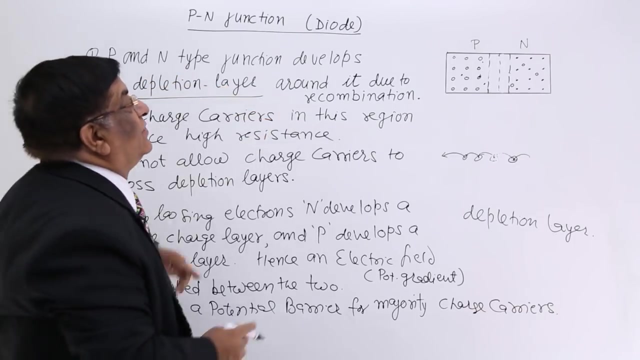 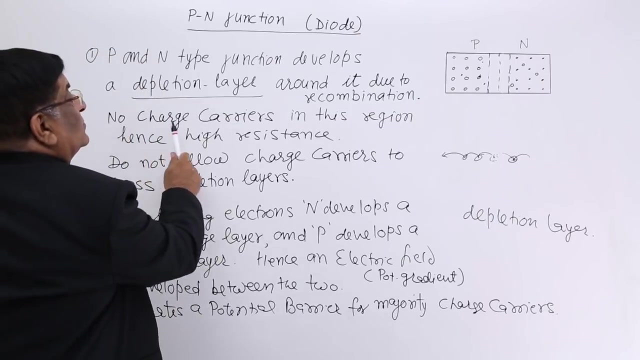 has been developed in this layer and because of that resistance the electrons are not able to move. ok, that is also correct. another thing here, see. ok, this is the first part i have written here. p and n type junction develop a depletion layer around it due to recombination- recombination of electrons and poles. no charge carrier in. 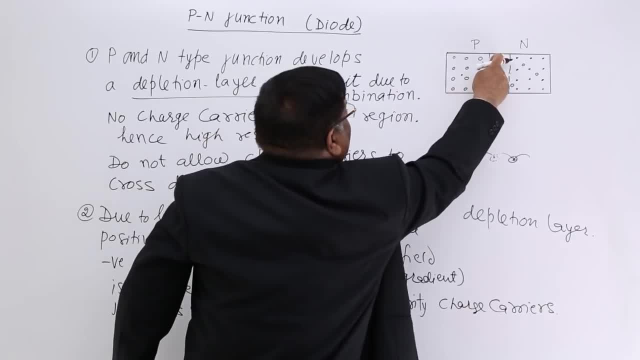 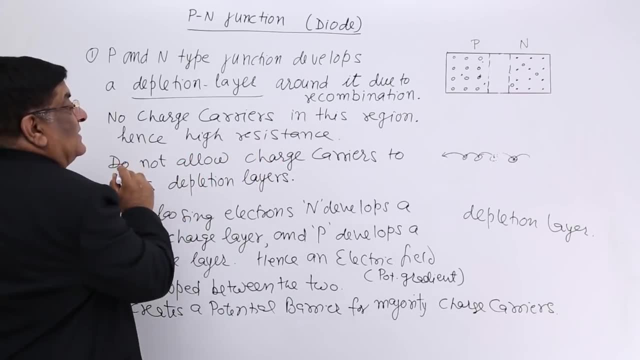 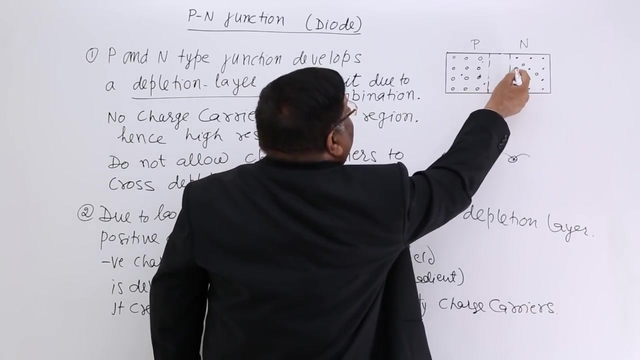 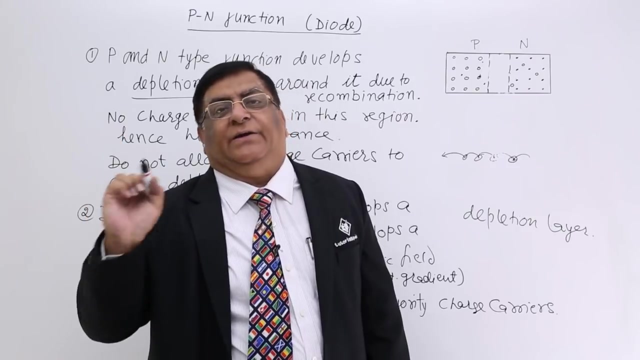 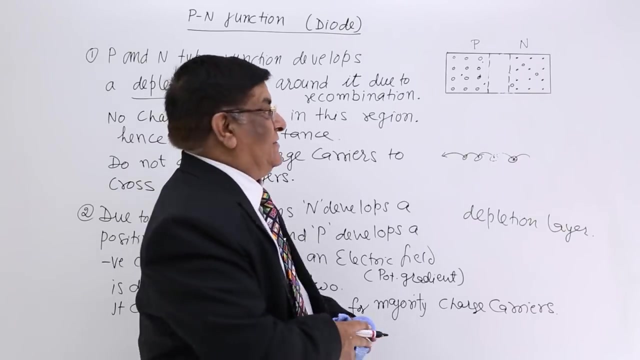 this region. there is no charge carrier in this region, hence it has high resistance. this do not allow charge carrier to cross depletion layer. these charge carriers now cannot cross this. you can say due to high resistance and due to lot of energy required to jump that, ok, energy per unit charge required is known as potential. right now see another thing here. 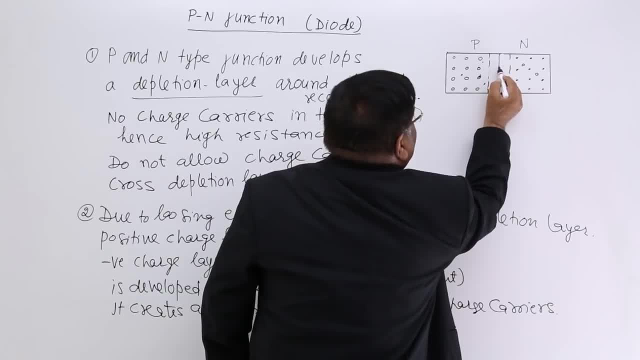 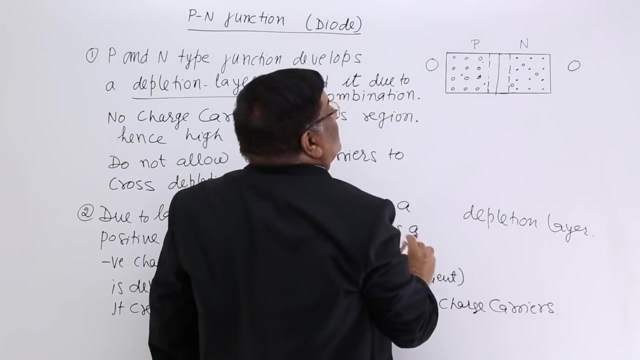 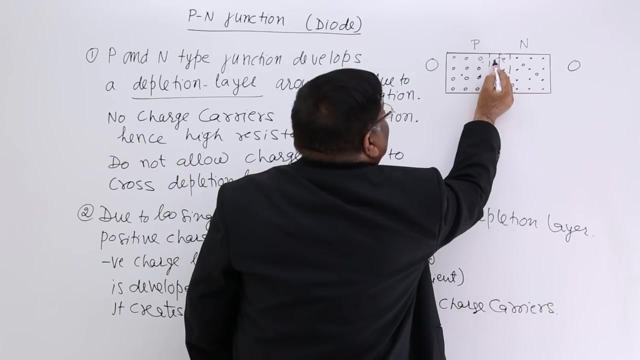 there were electrons. these electrons were part of n type semiconductor and they have gone here. what was the net charge of n type semiconductor? it was zero. what was the net charge of p type semiconductor? zero. from there, so many negative charges have left and gone here this way. if they have gone here, 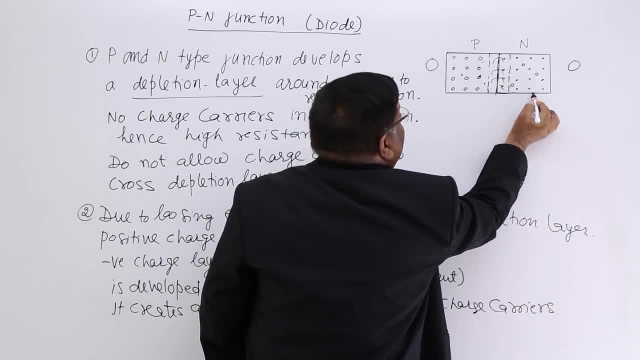 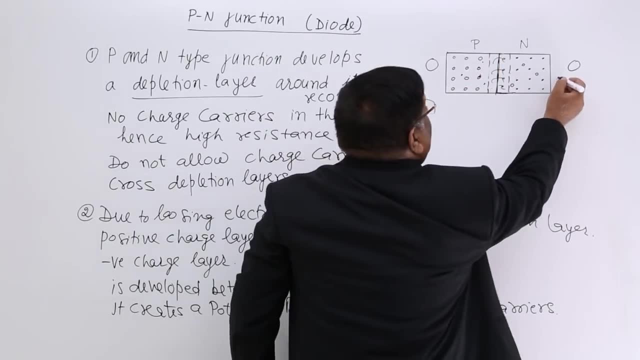 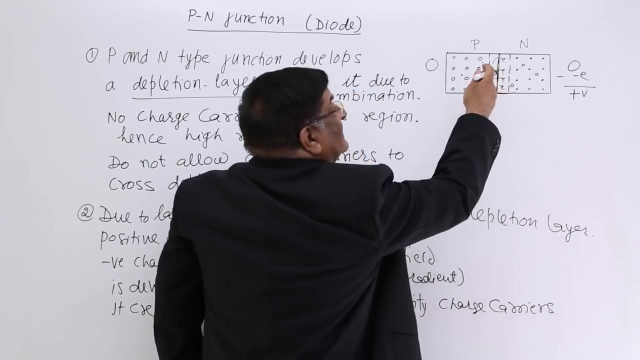 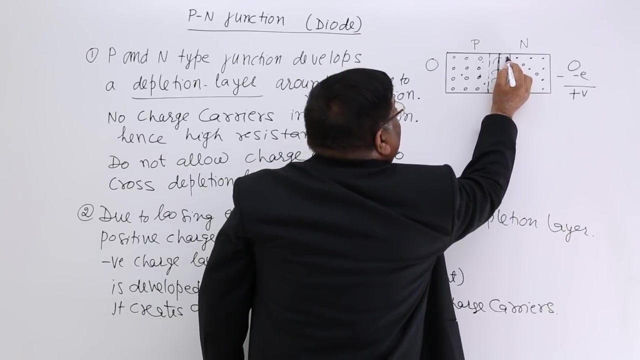 crossing this boundary. then what is the net charge of this semiconductor? this is the net charge of electron conductor. now, out of zero, negative has gone, so now it has become positive charge. so this develops positive charge where, at the location from where electrons have moved. so this develops positive charge here, because earlier the charge was zero. similarly, 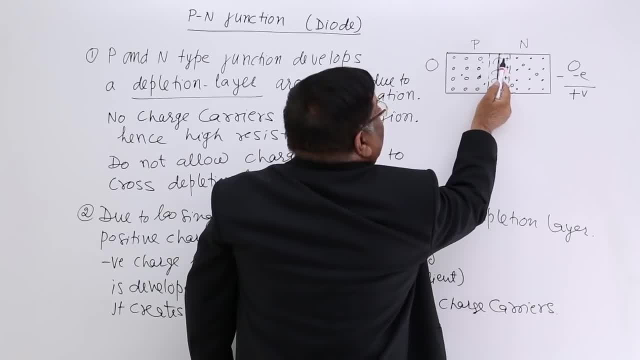 in p type earlier the charge was zero. when electrons moved the charge, i will say that the charge has cooling components- 붙ki here- and in p type earlier the charge has cooling seni, primary electrons, which actually becomes positive charge exercise. ask that from where electron has come here, electron here, electron here, electron here. If all these electrons 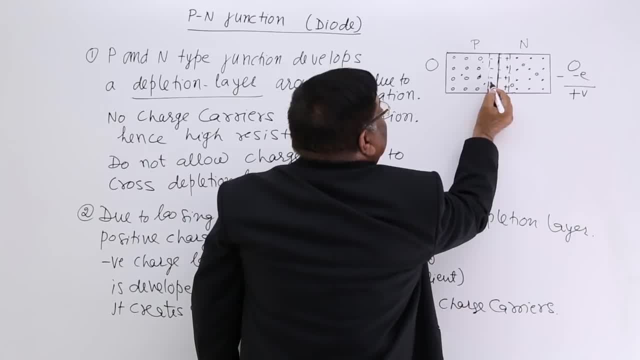 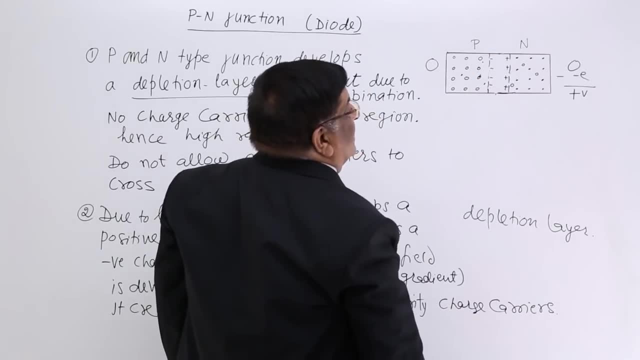 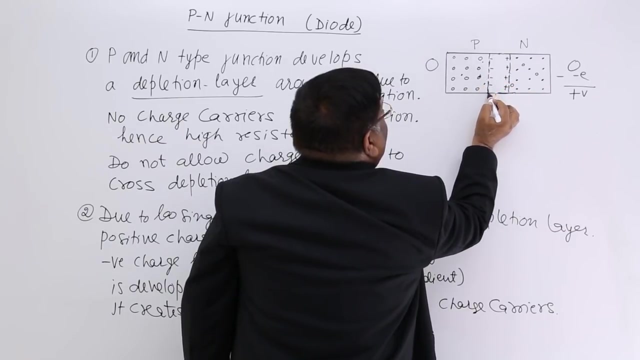 come here, here it develops minus, minus, minus, minus, And we see across the depletion layer. there is a positive surface here, there is a negative charge surface here, And this positive to negative charge surface, there is an electric field developed this way. This 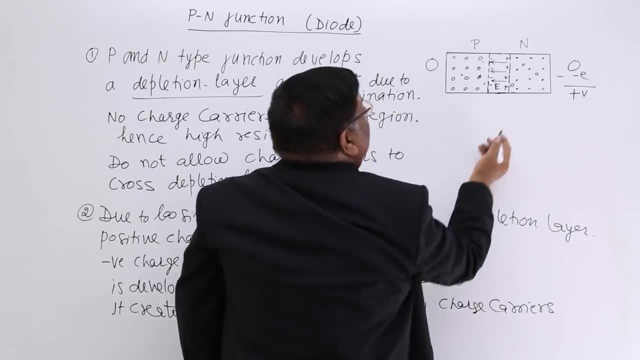 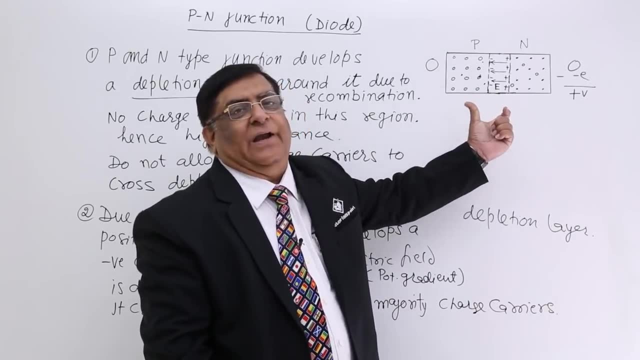 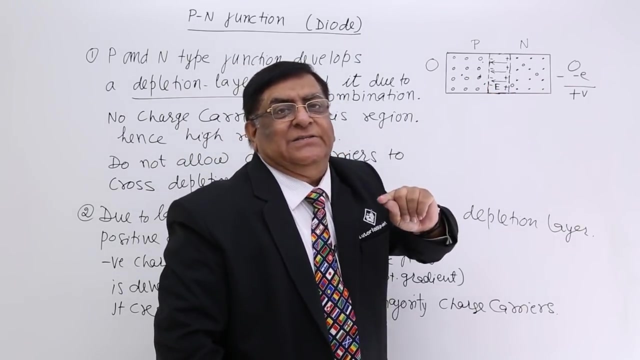 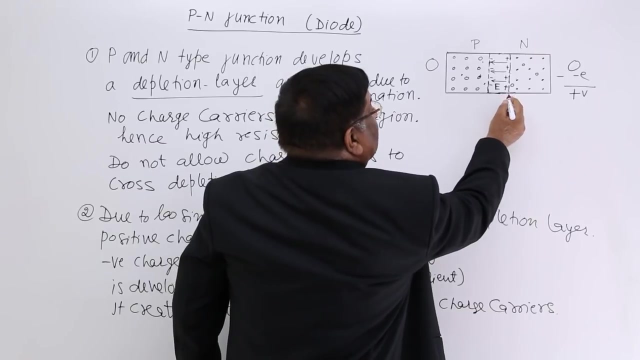 is electric field positive to negative charge. So in a p-n junction an electric field develops and there is certain distance. Electric field multiplied by distance is potential difference. hence there is a potential difference. If there is a potential difference here, this is positive potential, this is negative potential. 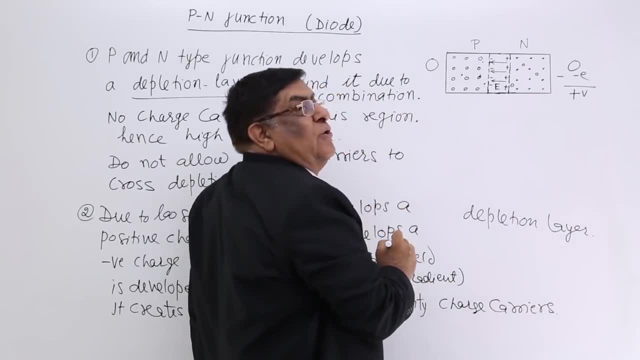 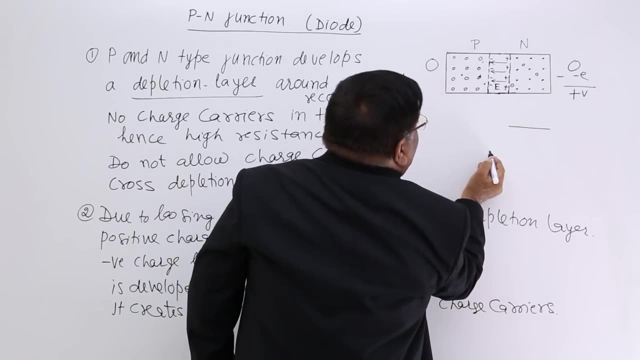 So this has got a higher potential, this has got a lower potential. Higher potential we denote by this level and this lower potential at this level. So we can say: this is the difference between potential of this layer and this layer. This is lower potential. 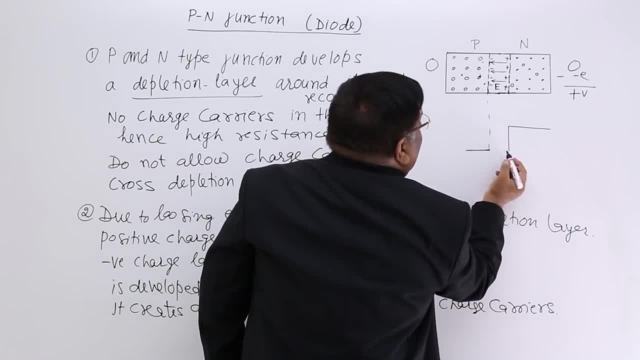 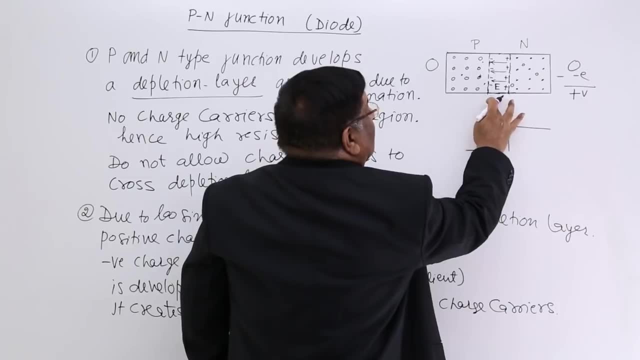 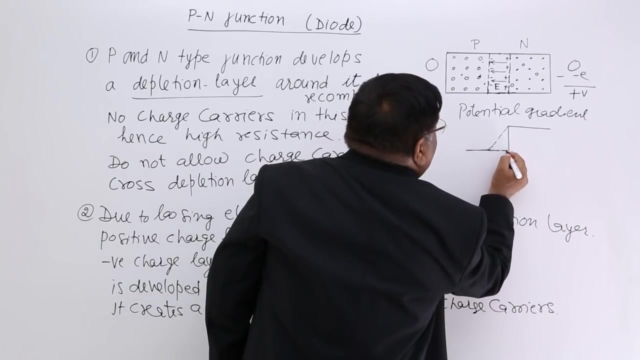 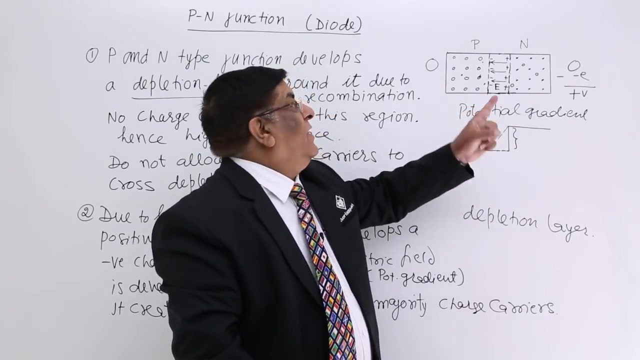 This is higher potential. And if we join the two this way, what is this? This is potential gradient, or electric field: Higher potential, lower potential. and what is this? This is difference of the potential: Lower potential, higher potential. Now a positive charge wants to. go here, Suppose, because there is a positive charge here, there is a negative charge here, So there is a positive charge here, there is a negative charge here, there is a negative charge here, So this is both positive and negative charge. 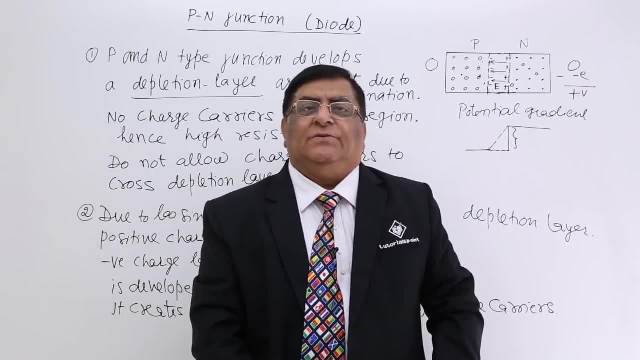 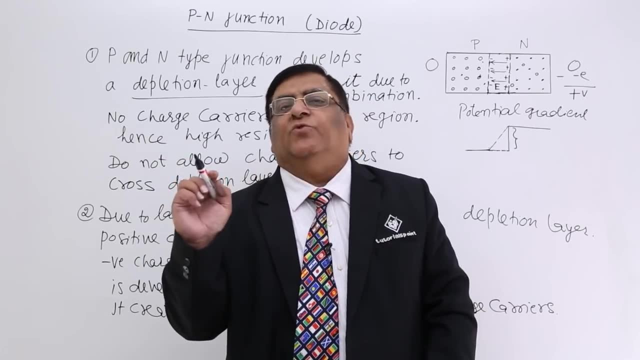 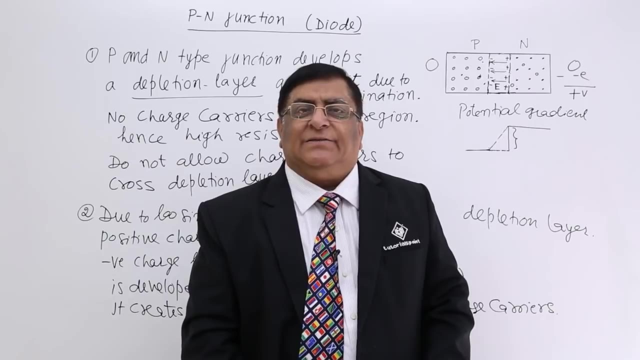 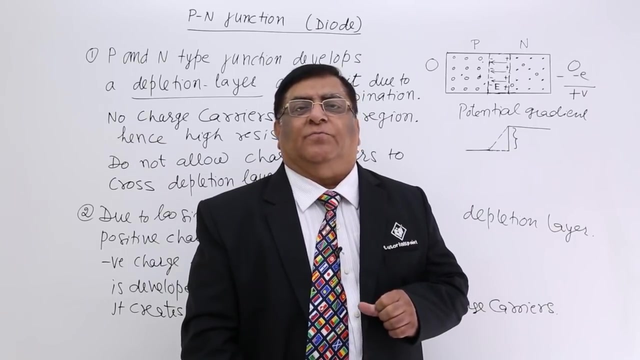 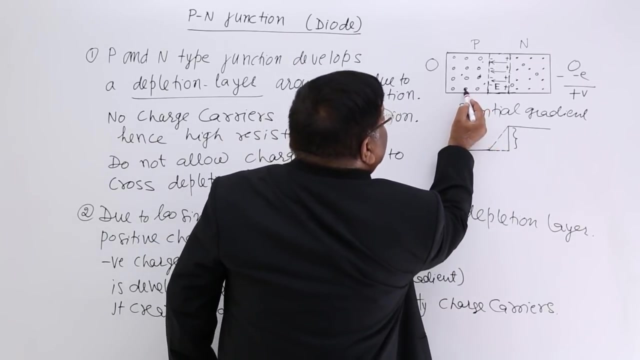 Because they are positive, we can say: positive charge is going off at this coming point Because, Well then, it is the vegetable gardeners children That is right. So this is the vegetable gardeners children. We make a vegetable garden to minus. And here you see, these are positive charges, positive positive and voltage is. 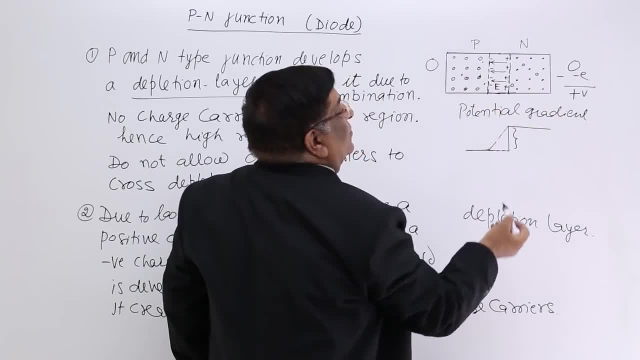 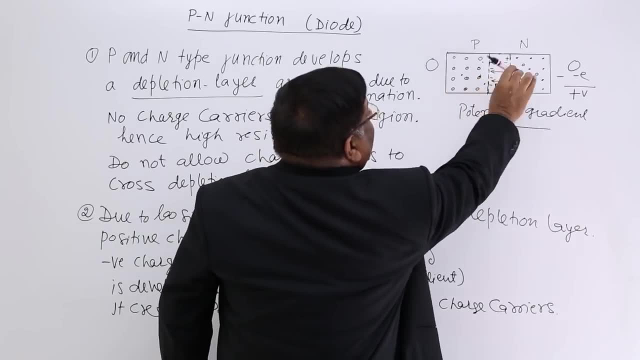 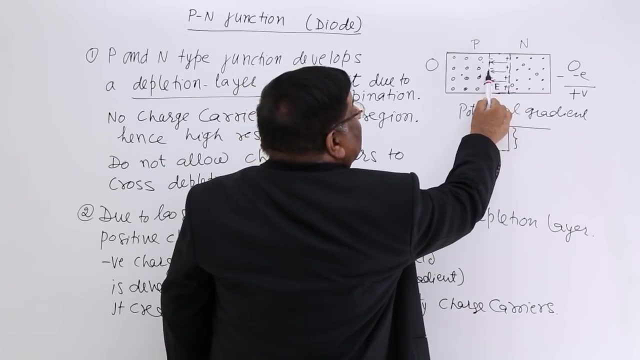 like this. Can it go and jump here? Answer is no. These are electrons. What is the tendency of electron? to go from minus to plus. Minus to plus, but they cannot go plus to minus. that will oppose them. Therefore, these electrons are restricted by this potential difference. 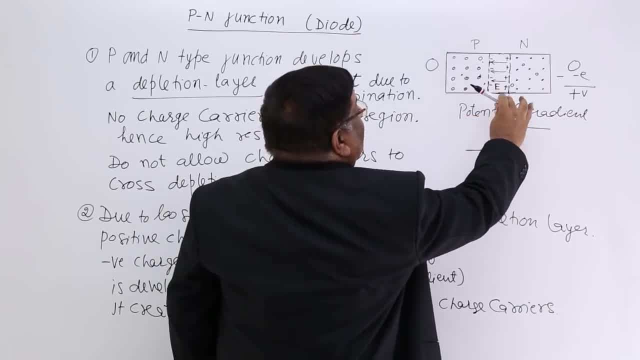 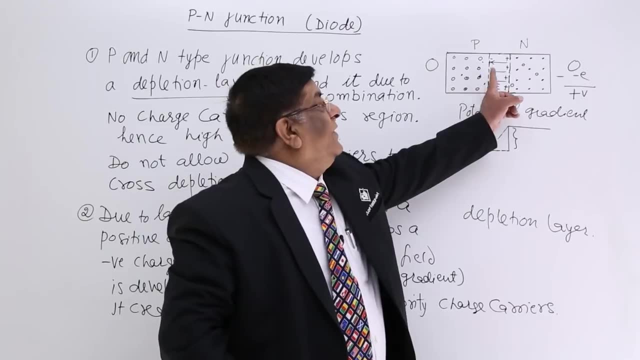 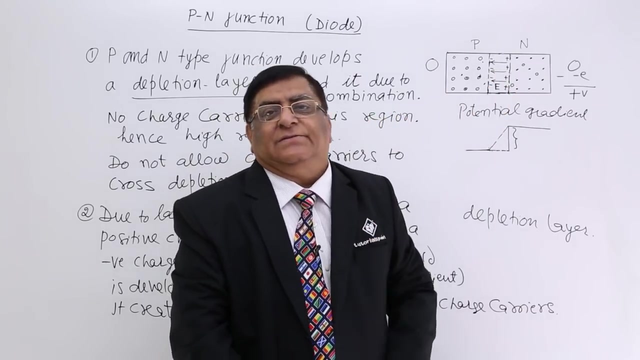 and these holes are restricted by this potential difference because that is in opposite direction. Now, if a positive hole want to go here, it should have an energy, much more energy than this potential difference. Otherwise it cannot go, because this potential is blocking the 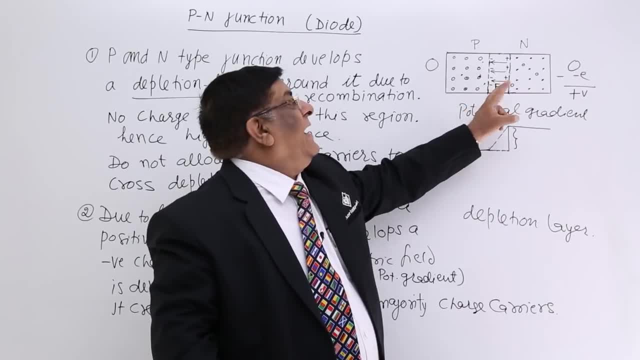 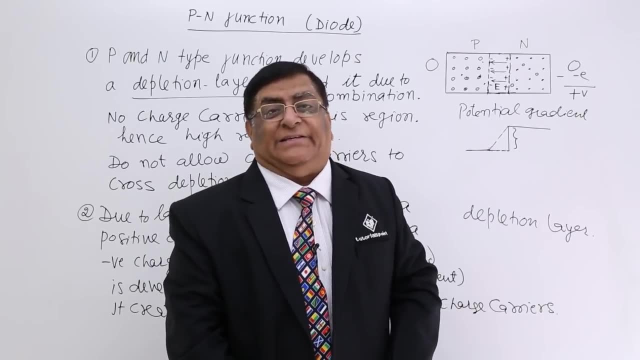 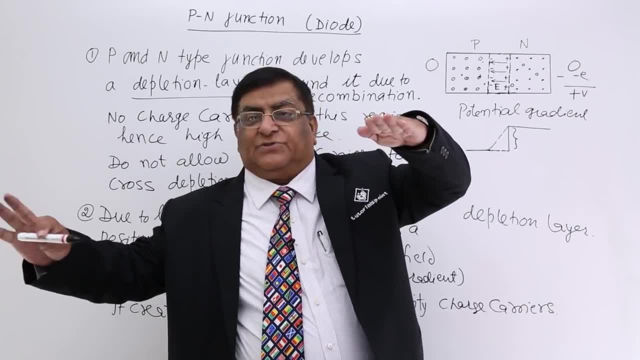 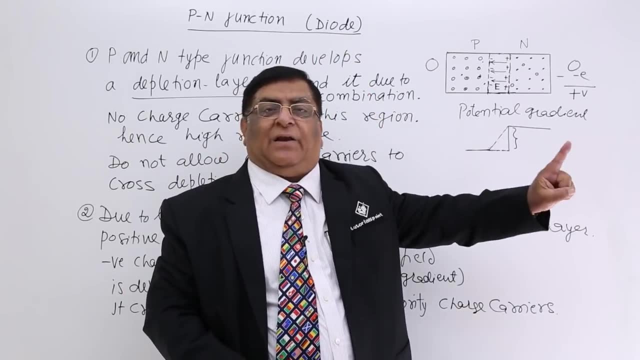 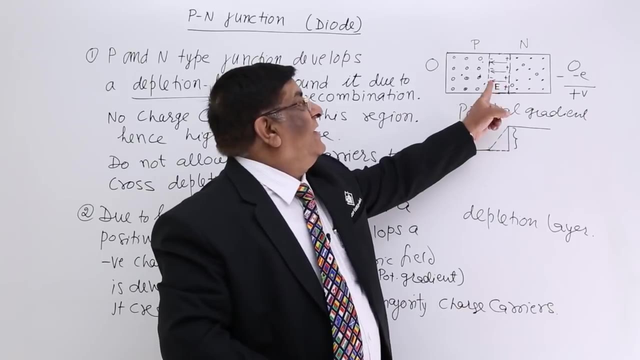 Barrier, because if a positive charge come from here, it has to be jumped. because it cannot jump, It will remain on this side. Similarly, an electron is coming from here, It has to jump it. The barrier is in between. So this potential difference. 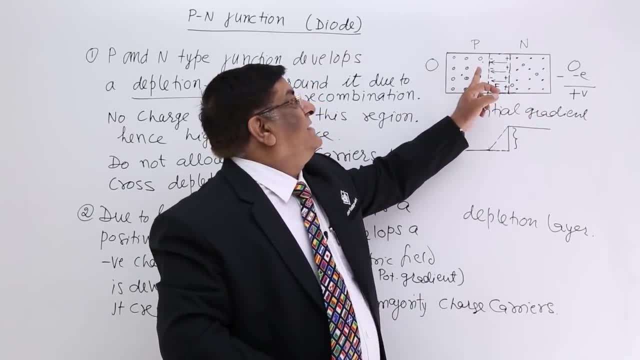 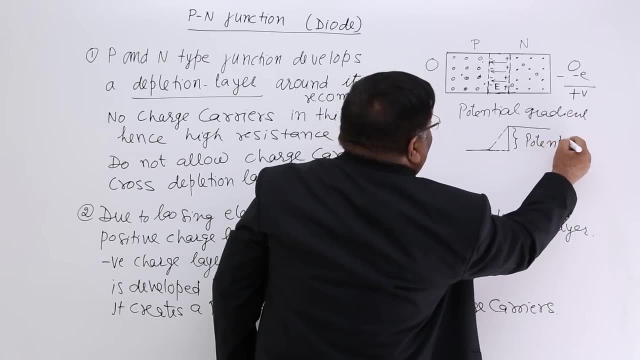 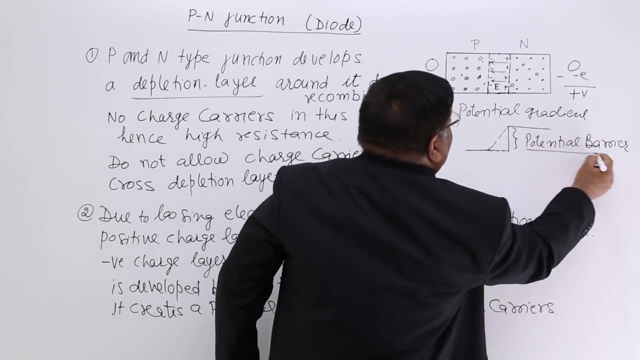 becomes between electrons are not allowed to go here. these are not allowed to go here. so this wall is known as potential barrier. whatever is the potential difference between the two, that is the value, or that is the height of potential barrier. this height, it is known. 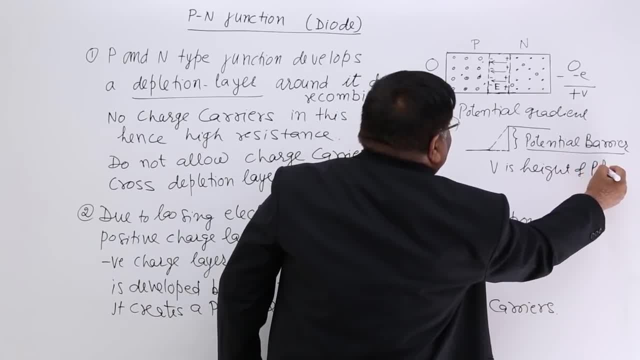 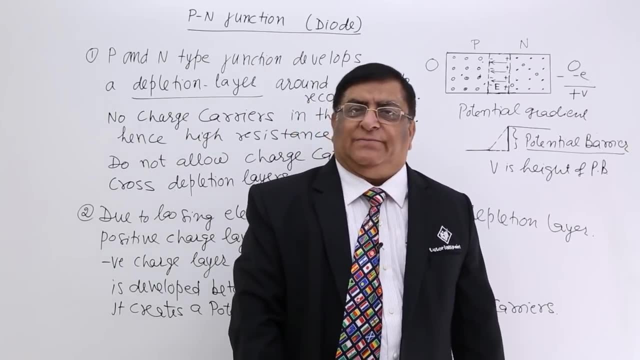 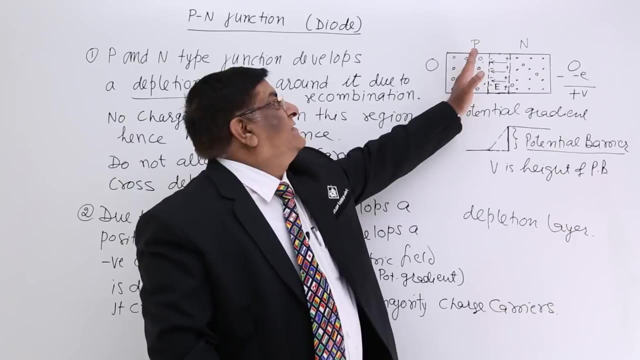 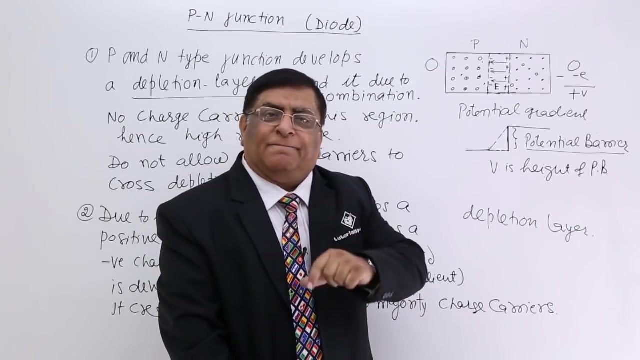 as height of potential barrier. this, what is potential energy? work done? so much work has to be done on it if it wants to cross and it does not have that much energy. so this remain here. this remain here. so majority charge carrier cannot pass through now this thing. 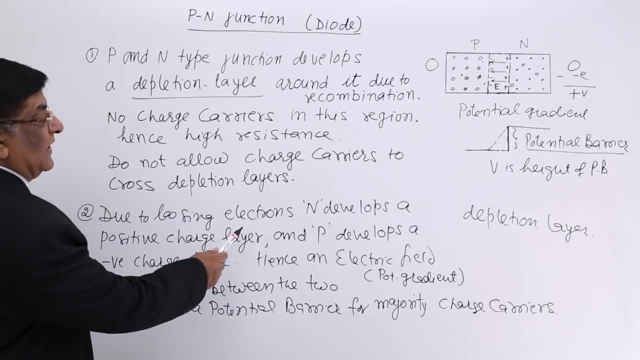 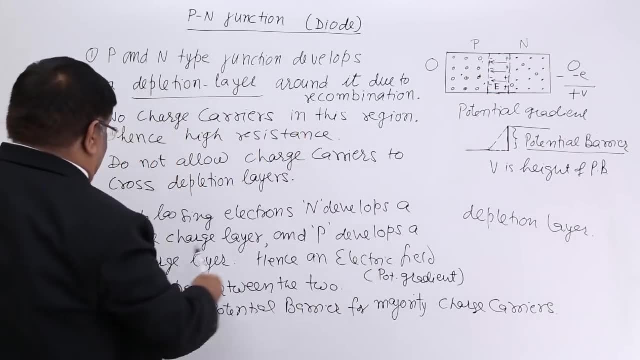 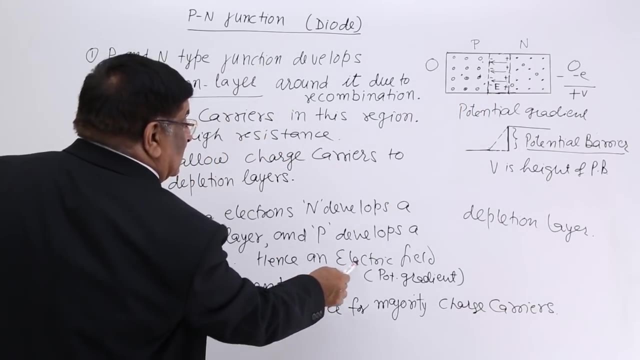 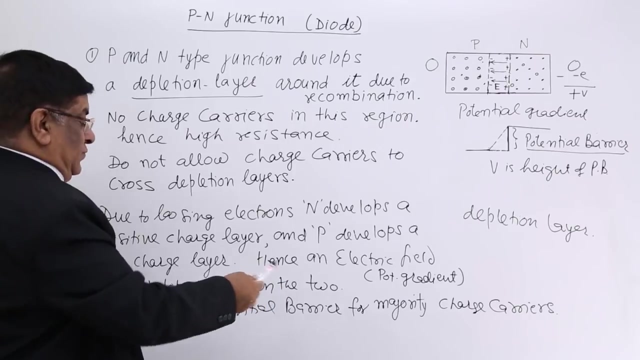 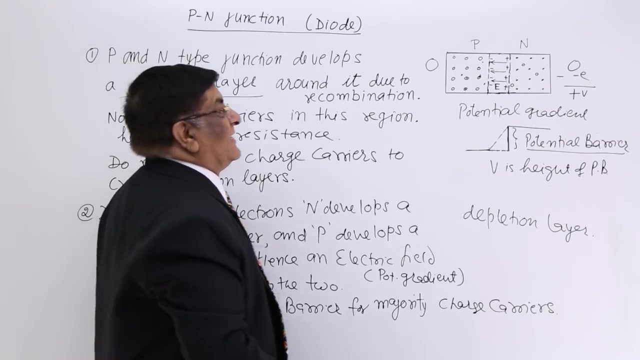 we have written here, due to losing electrons and type, develops a positive charge layer and p develops a negative layer. here, hence, on, an electric field is developed, that is, potential gradient is developed between the two. it create a potential barrier for majority charge carrier. a direction is such that it creates a barrier. 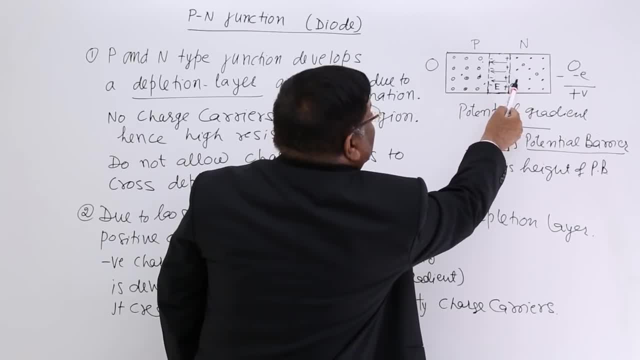 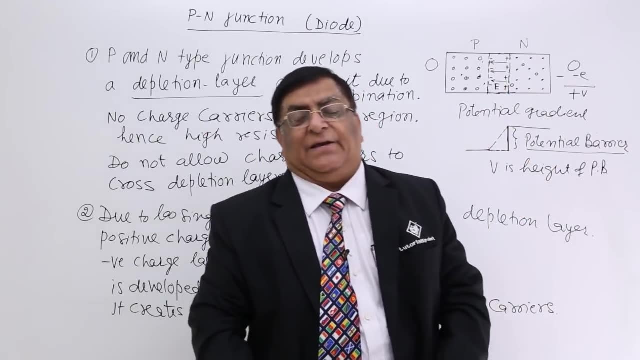 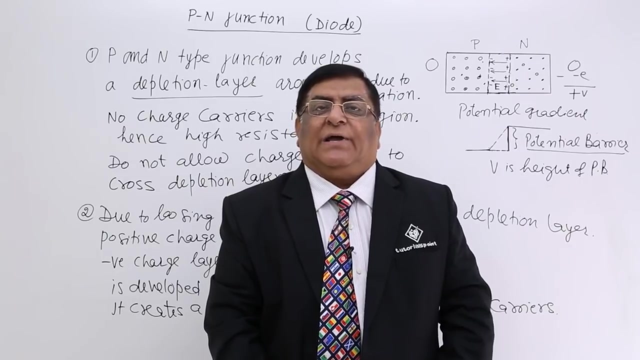 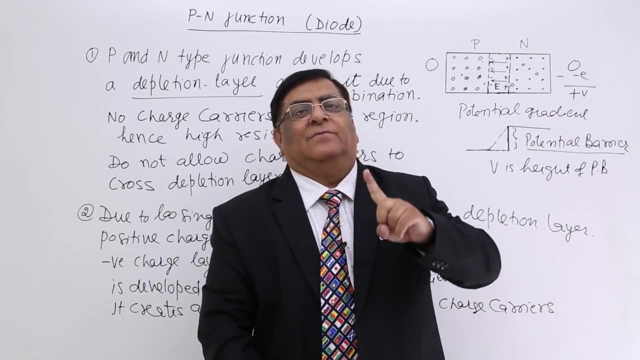 these are not allowed to go here and these negative are not allowed to go here. so this creates a barrier and because of this barrier, they stopped recombining each other. so this is what happens when we make a pn junction: a layer is created and potential barrier is. 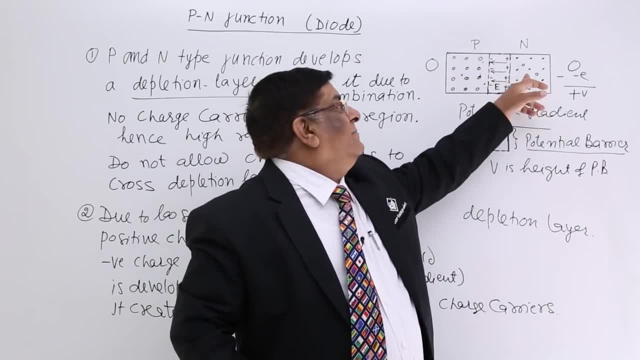 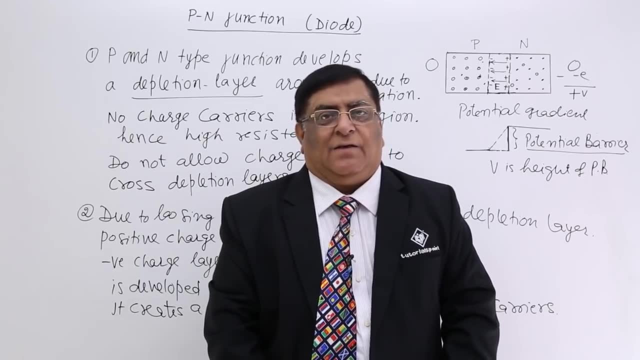 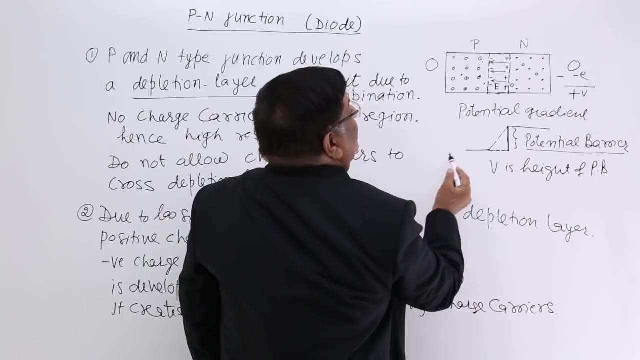 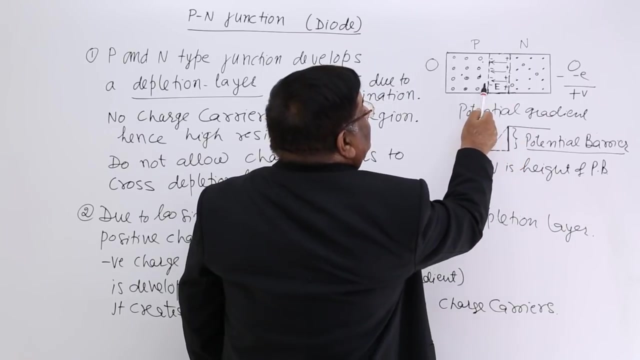 created. majority charge carrier blocked here. majority charge carrier is blocked here. majority charge carrier blocked here. what happens to minority charge carrier? well, minority charge carriers are allowed. how. what is minority charge carrier here negative? and this potential difference is this way: negative can move from minus to plus, so this moves here and very. 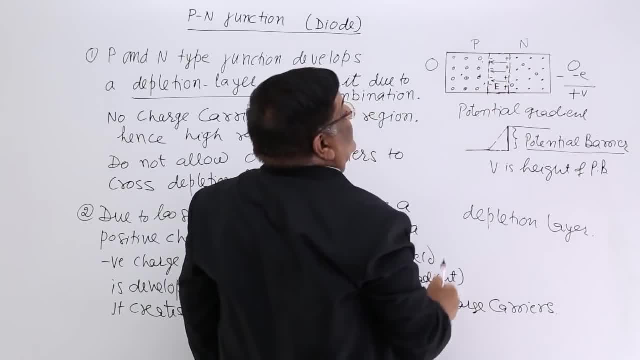 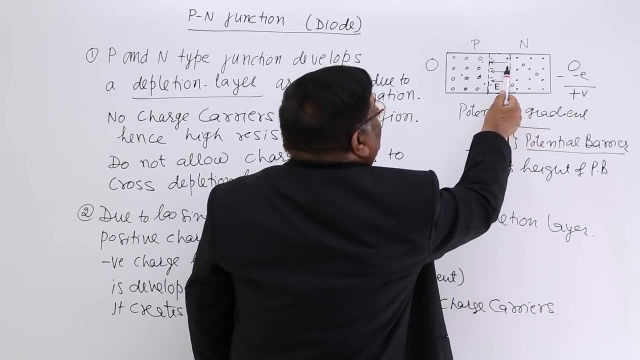 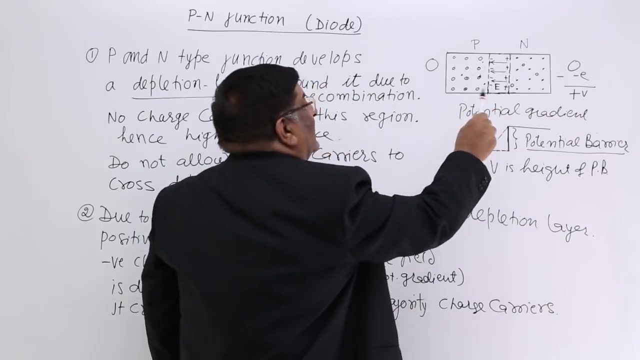 easily go to n type and recombine with this. similarly, this whole pn junction is blocked. they are allowed to move from plus to minus. so they move from plus to minus if they are close by the surface like this. it will move here, it will move here and this will recombine. 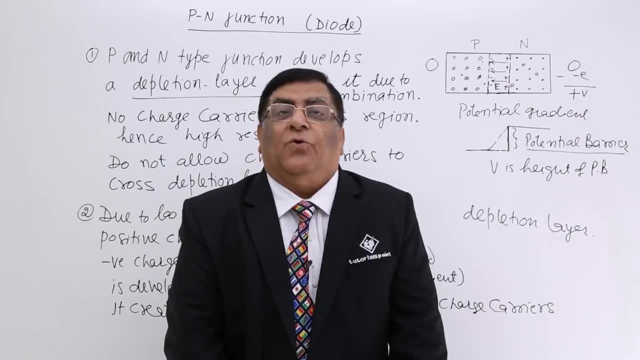 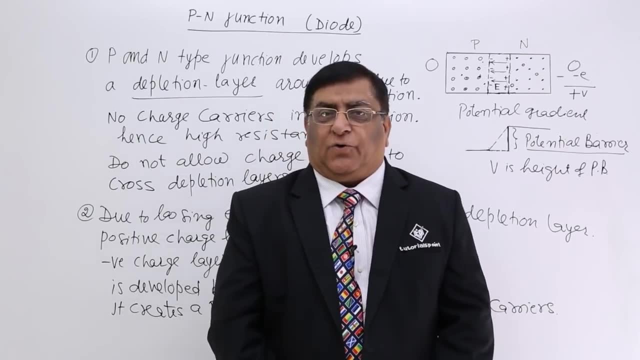 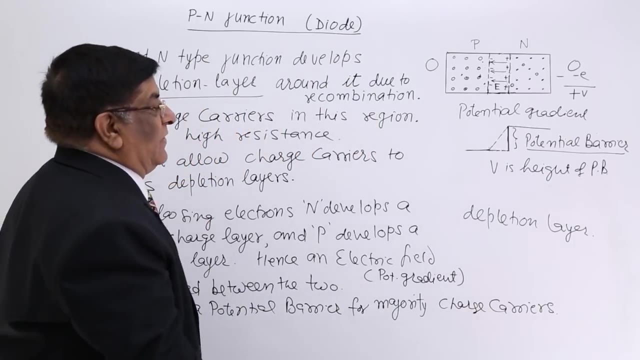 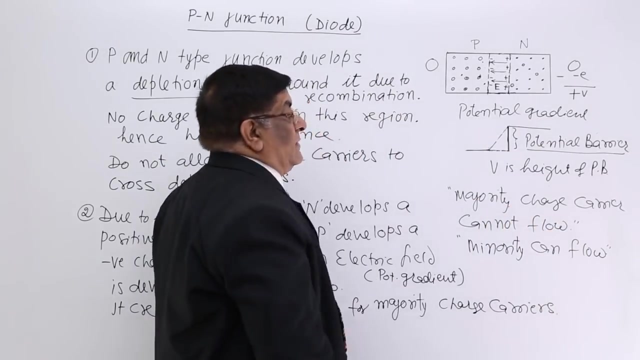 so minority charge carriers can flow through a potential barrier. who cannot flow? majority charge carrier cannot flow. minority charge carrier can very well flow. they can form a correct so that we will know that this is a potential barrier. so this is a potential barrier. so we will note here: majority charge carrier cannot flow, minority can flow and they flow. 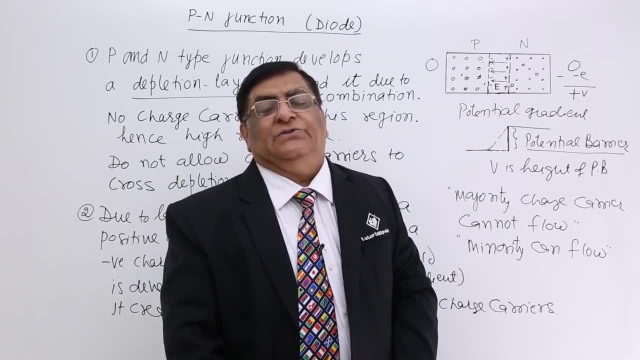 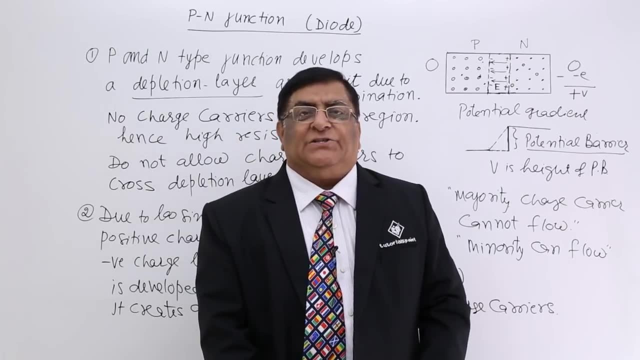 for sometime, till they are settled. so this way, this is the action of pn junction. so in pn junction, what is created? a deflation layer, a potential barrier which do not allow charge carrier to go, and what is the potential barrier that can happen in pn junction order? now let's 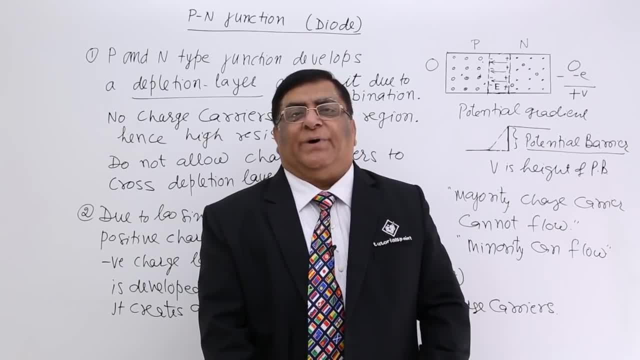 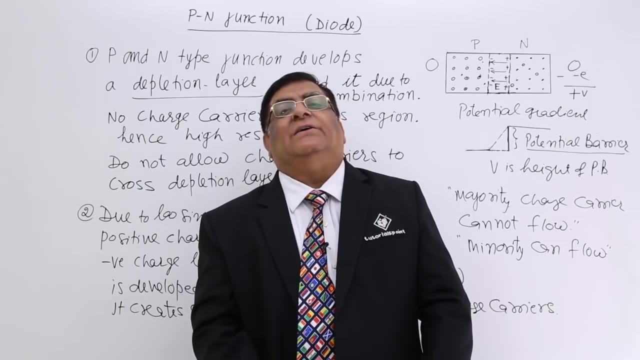 to pass. if this does not allow charge carrier to pass, what can we comment about? whether it is an insulator or it is a conductor? the answer: because it does not allow charge particle to pass over, then it behaves like a insulator. it will not allow the current to pass, whatever.